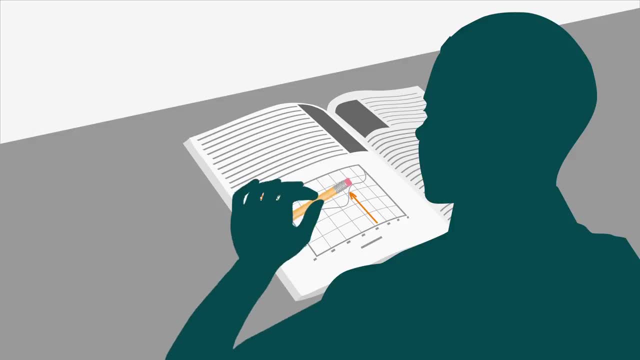 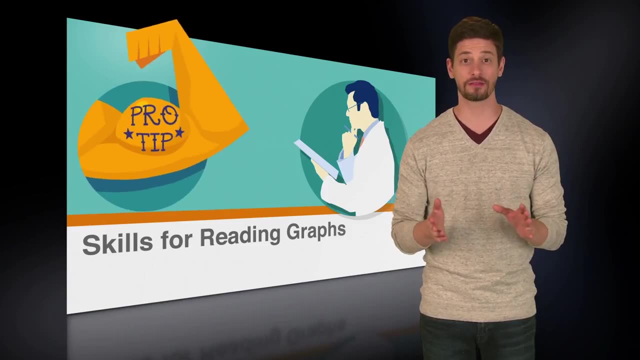 so that you can find the values more quickly and easily. Use your pencil to help you draw vertical and horizontal lines to enable more accurate reading. Here's a pro tip: When you're reading graphs, be sure to pay attention to the labels of the axes and the scales of measure. They may not 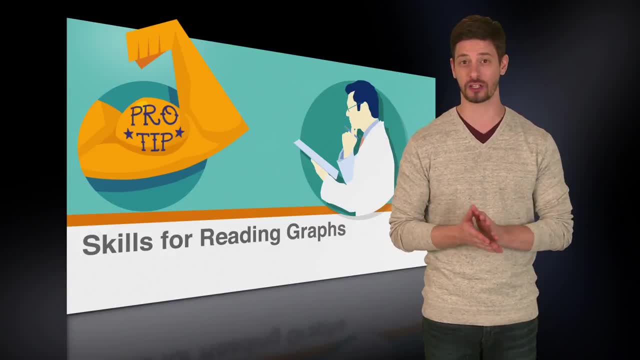 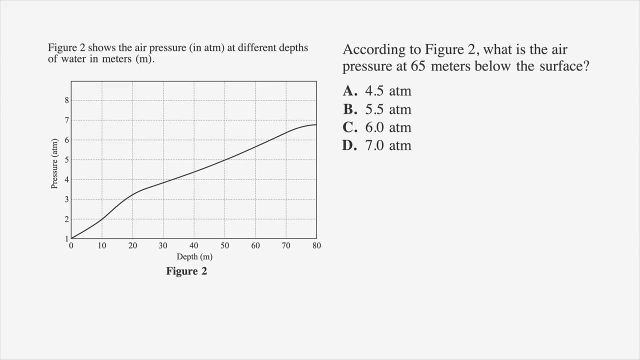 be set up the way you would expect, and you don't want to be able to see them. So if you're reading a graph, you might want to use the wrong information. With that in mind, let's take a look at a question based on a graph. According to Figure 2,, what is the air pressure at 65 meters? 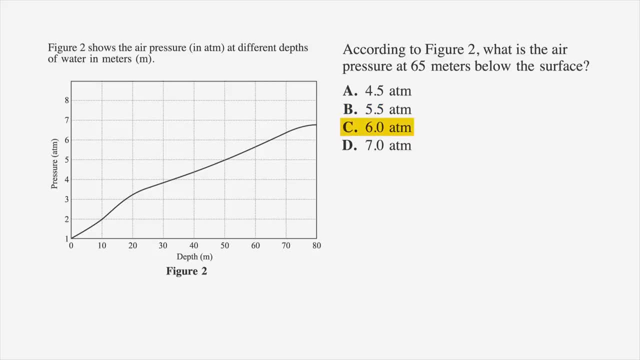 below the surface. The answer choices are A- 4.5 atm, B- 5.5 atm, C- 6.0 atm and D- 7.0 atm. To answer this question, look at Figure 2.. Note where the units of measure are located on the graph. 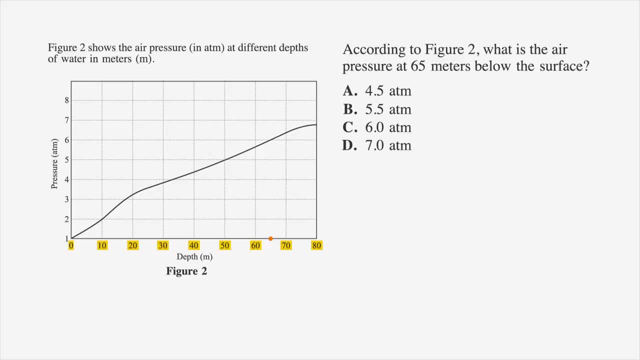 axis, which represents depth. This is an example of how a graph can sometimes look counterintuitive because you might expect the depth to be represented vertically. Use your pencil to follow this point up until you reach the line on the graph. Now draw a line to the left, using your second pencil if necessary. 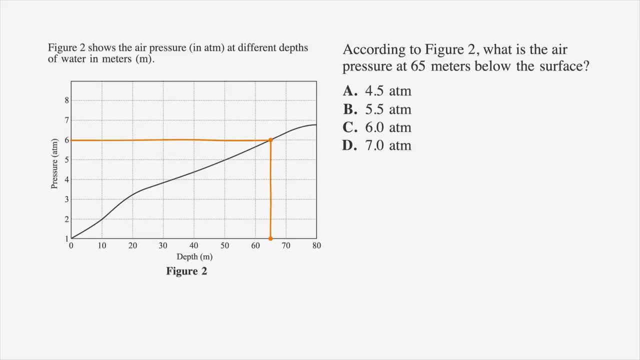 until you reach the y-axis, which represents pressure. The point you reach on the y-axis should be 6.0 atmospheres, which means that at a depth of 65 meters below the surface, the pressure is 6.0 atmospheres. We have our answer: choice C. 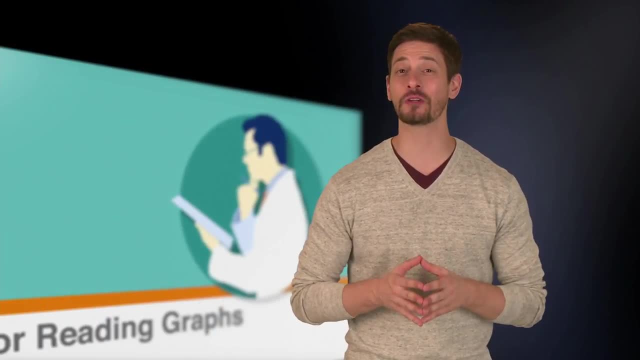 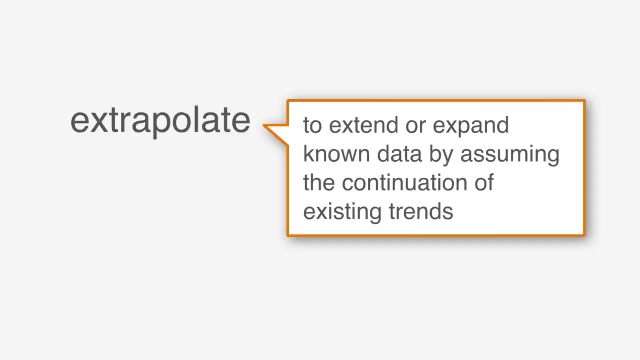 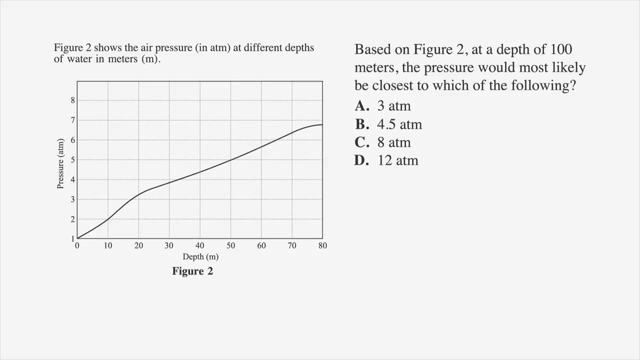 Another skill that you'll be tested on is your ability to extrapolate based on the information you have. Extrapolate means to extend or expand known data by assuming the continuation of existing trends. Let's look at an example based on the same graph, Based on figure 2. at a depth of 100 meters, the pressure would 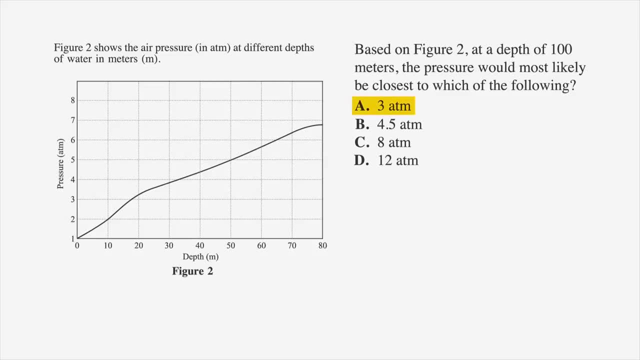 most likely be closest to which of the following: Choice A is 3 atmospheres, choice B is 4.5 atmospheres, choice C is 8 atmospheres and choice D is 12 atmospheres. When you look at the graph, you'll see that it. 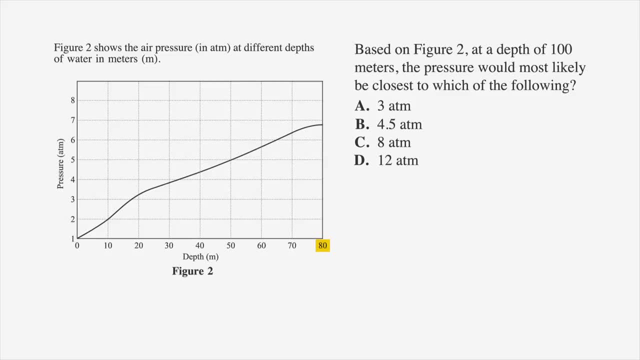 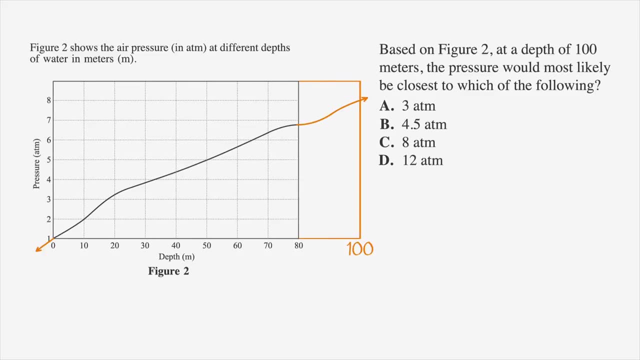 represents depths no greater than 80 meters, so you'll need to extrapolate to find the closest value. You can take out your pencil and extend the line to where it would logically fall on the graph at a depth of 100 meters. Draw your line to.